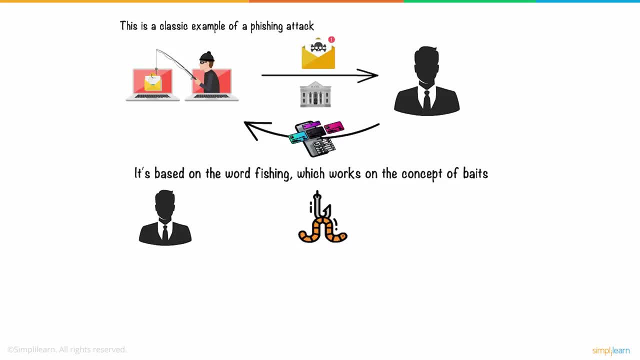 of baits. if a supposed victim catches the bait, the attack can go ahead, which, in our case, makes jane the fish and the phishing emails the bait. if jane never opened the malicious link or was cautious about the email authenticity, an attack of this nature would have been relatively ineffective. 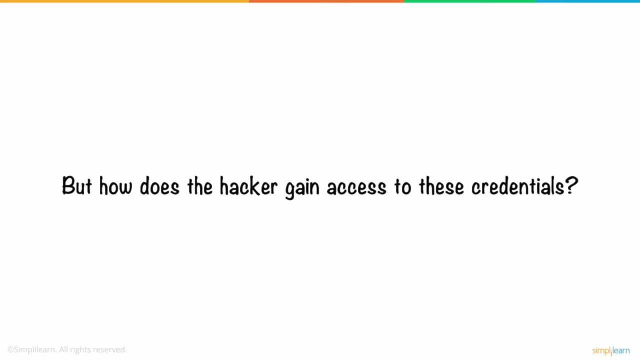 but how does the hacker gain access to these credentials? a phishing attack starts with a fraudulent message which can be transmitted via email or chat applications, even using sms conversations. to impersonate legitimate sources is known as smishing, which is a specific category of phishing attacks. irrespective of the manner of transmission, the message targets the victim. 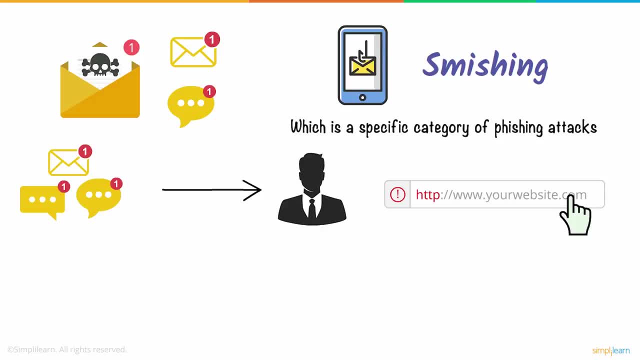 in a way that coaxes them to open a malicious link and provide critical information on the record of the attack. the phishing attack can be transmitted via email or chat applications website. more often than not, the websites are designed to look as authentic as possible once the victims submit information using the link, be it a password or credit card details. 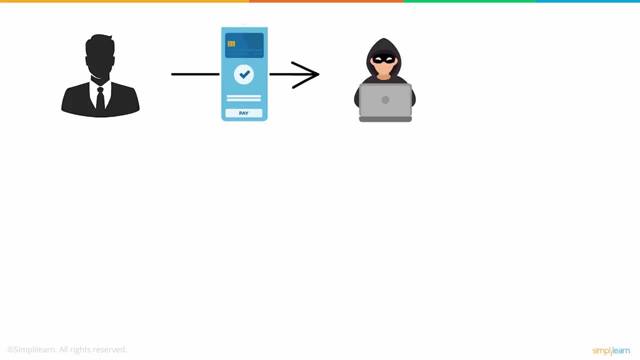 the data is sent to the hacker who designed the email and the fake website, giving him complete control over the account whose password was just provided. often carried out in campaigns where an identical phishing mail is sent to thousands of users, the rate of success is relatively low, but 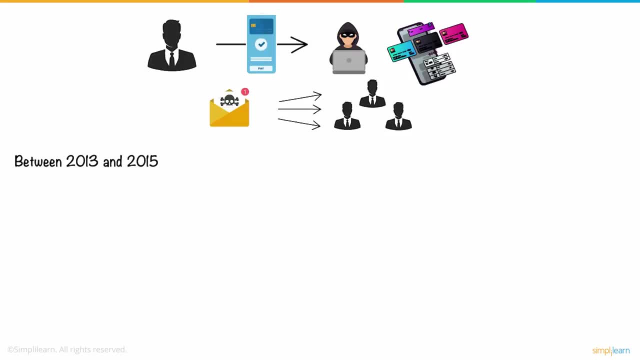 never zero. between 2013 and 2015, corporate giants like facebook and google were tricked off of 100 million dollars due to an extensive phishing campaign where a known common associate was impersonated by the hackers. apart from credit access, some of these campaigns target the victim. 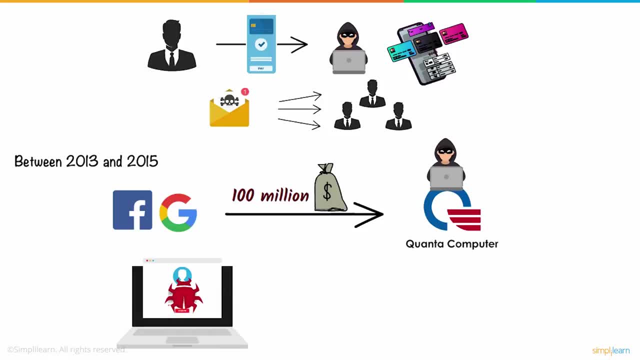 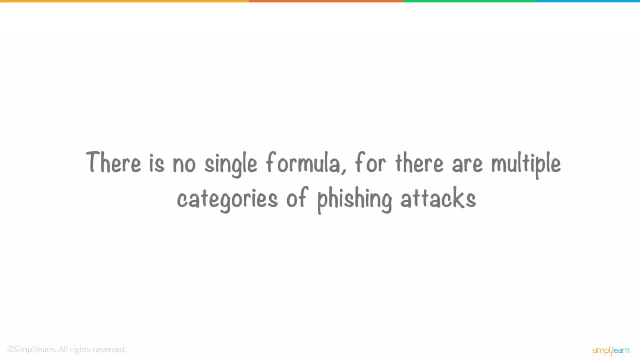 device and install malware when clicked on the malicious links, which can later function as a botnet or a target for ransomware attacks. there is no single formula for there are multiple categories of phishing attacks and there is no single formula for there are multiple categories of phishing attacks. 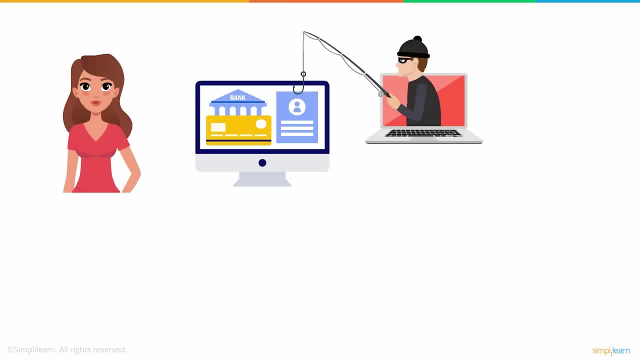 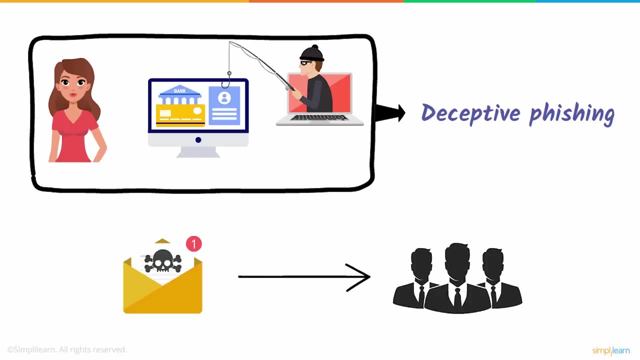 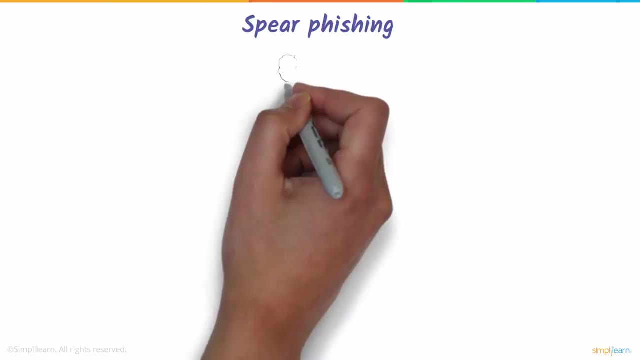 the issue with jane, where the hacker stole her bank credentials, falls under the umbrella of deceptive phishing. a general email is sent out to thousands of users in this category, hoping some of them fall prey to this scam. spear phishing, on the other hand, is a bit customized version. the targets are: 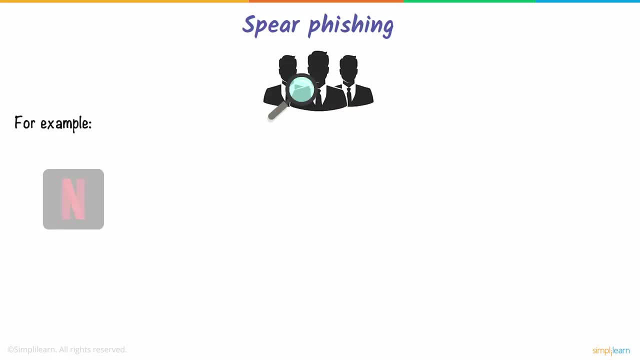 researched before being sent an email. for example, if you never had a netflix subscription, sending you an email that seems like the netflix team sends it becomes pointless. this is a potential drawback to phishing attacks of deceptive phishing techniques. on the other hand, a simple screenshot of a spotify playlist. 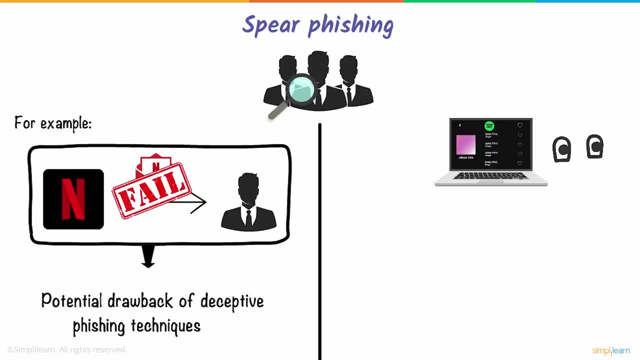 being shared on social media indicates a probable point of entry. the hacker can send counterfeit messages to the target user while implying the source of such messages being spotify, tricking them into sharing private information. since the hacker already knows the target uses spotify, the chances of victims taking the bait increase substantially. 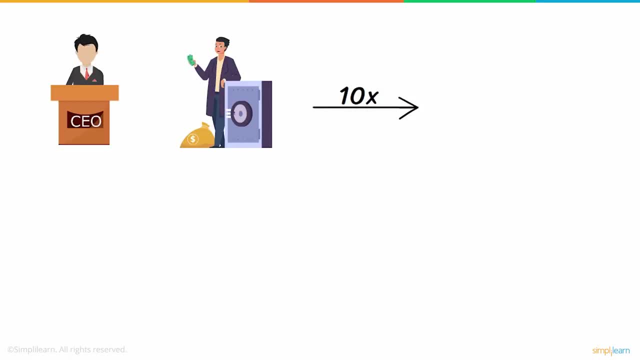 for more important targets, like ceos and people with a fortune on their back. the research done is tenfold, which can be called a case of whaling. the hackers prepare and wait for the right moment to launch their phishing attack, often to steal industry secrets for rival companies. 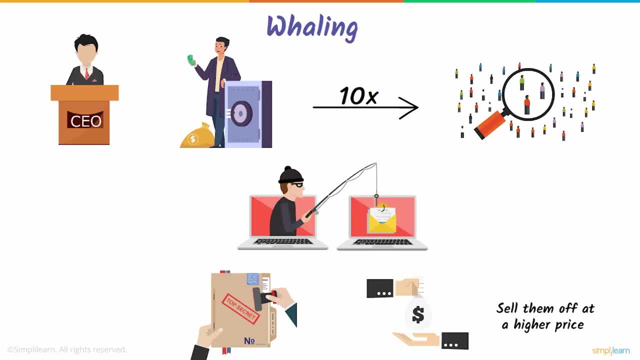 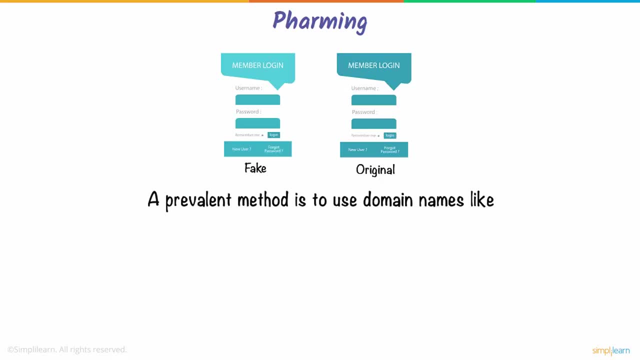 or sell them off at a higher price. apart from just emails, farming focuses on fake websites that resemble their original counterparts as much as possible. the prevalent method is to use domain names like facebook with a single o or youtube with no e. these are mistakes that people make. 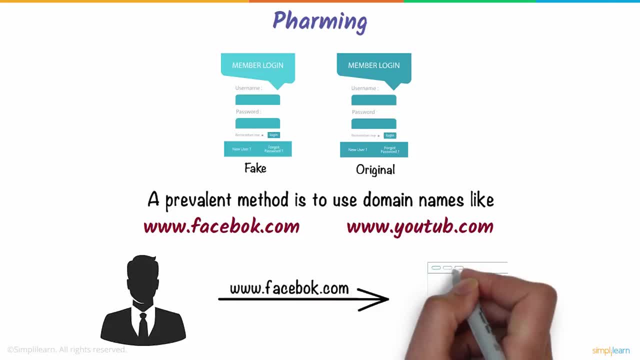 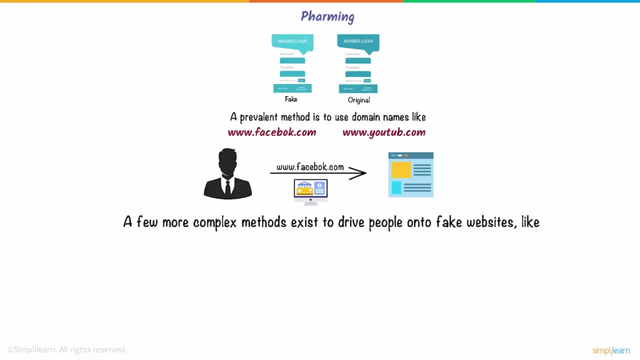 when typing the full url in the browser, leading them straight to a counterfeit webpage which can fool them into submitting private data. a few more complex methods exist to drive people onto fake websites, like arp spoofing and dns cache poisoning, but they are rarely carried out due to time and 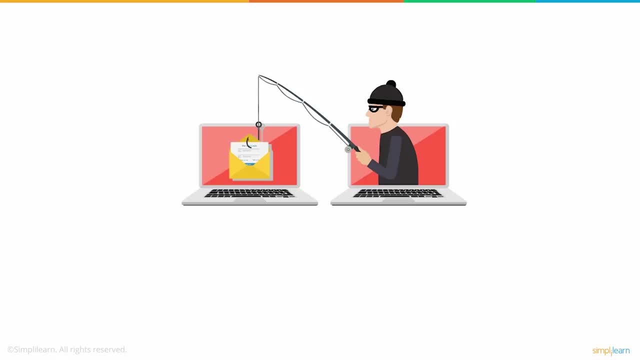 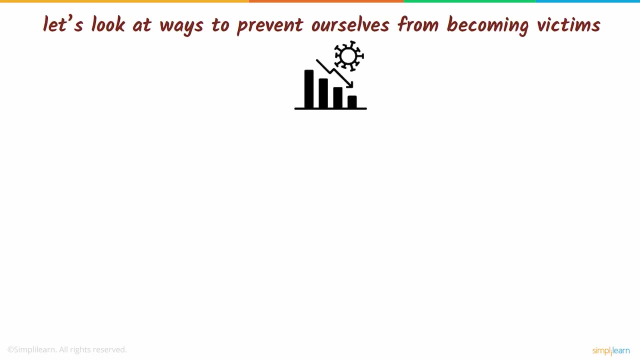 resource constraints. now that we know how phishing attacks work, let's look at ways to prevent ourselves from becoming victims. while the implications of a phishing attack can be extreme, protecting yourself against these is one of the most important aspects of phishing attacks. relatively straightforward, jane could have saved herself from credit card fraud had she checked. 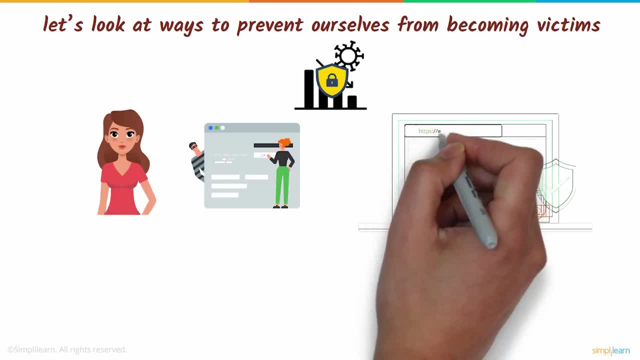 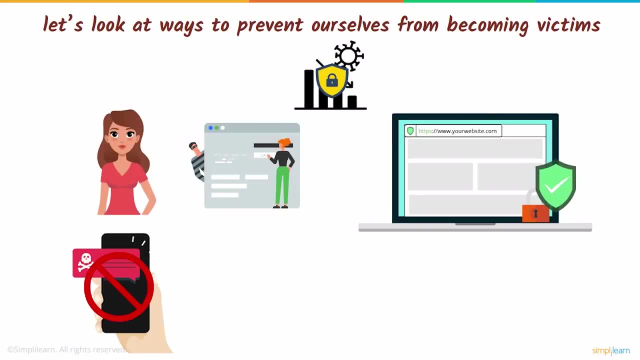 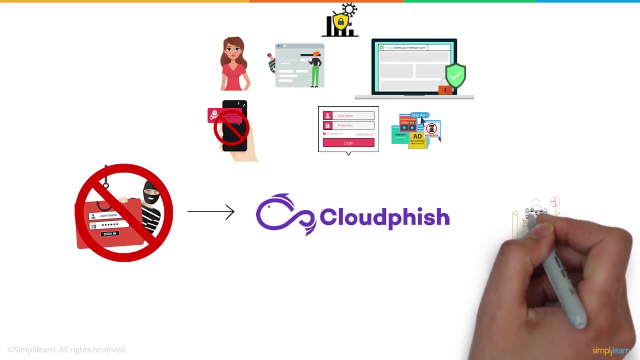 the link in the email for authenticity and that it redirected to a secure website that runs on the https protocol. even suspicious messages shouldn't be entertained. one must also refrain from entering private information on random websites or pop-up windows, irrespective of how legitimate they seem. it is also recommended to use secure anti-phishing browser extensions like cloudfish to sniff out. 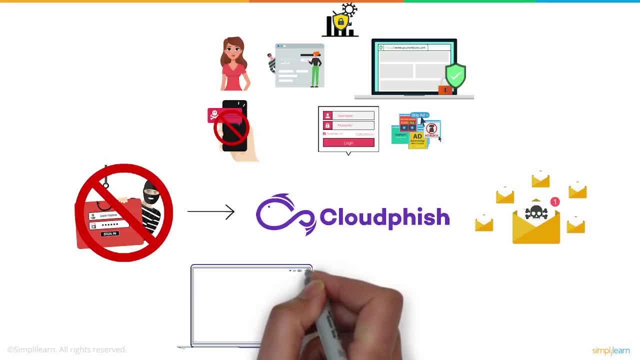 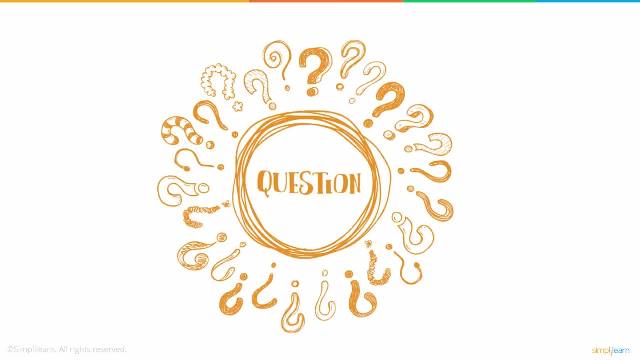 malicious emails from legitimate ones. the best way to prevent phishing is browsing the internet with care and being on alert for malicious attempts at all times. so here is a question for you: if both me and my friends receive the same email that instructs us to change our spotify password,